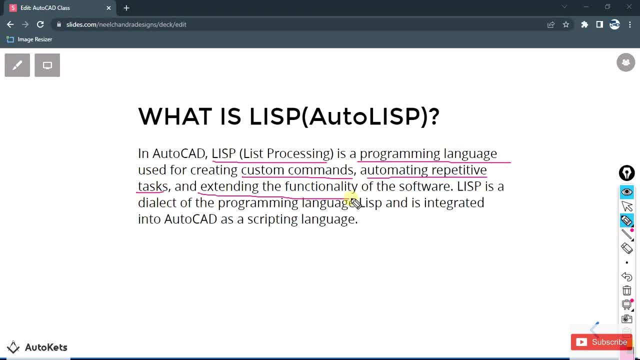 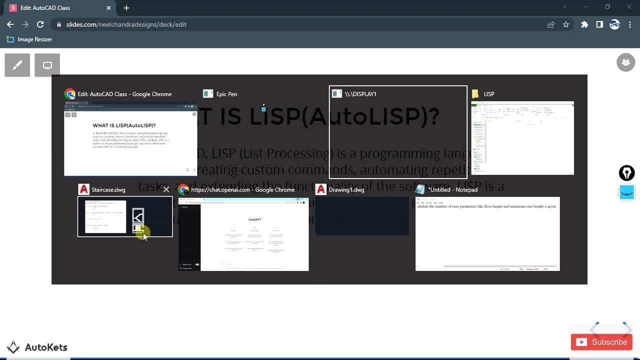 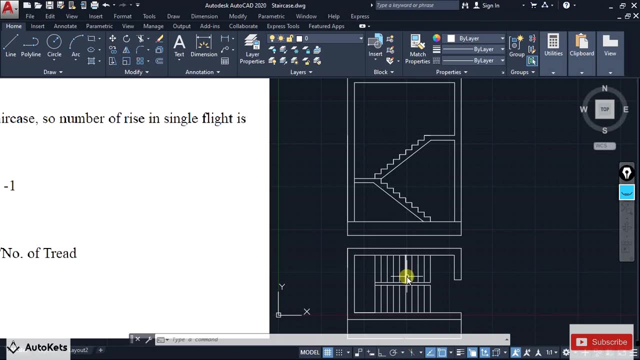 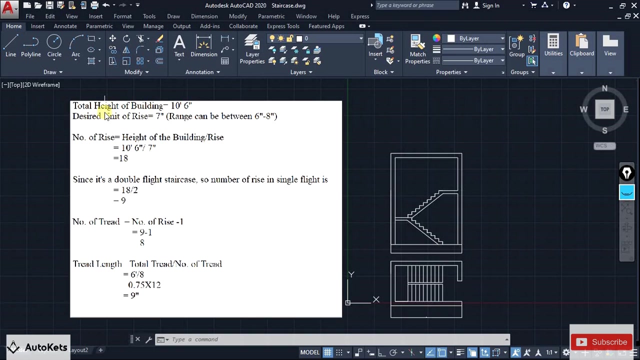 creating the custom commands and these operations. So let's just see how to create the list file. So I have one. I am going to start my AutoCAD And here you can see that I have created a staircase. And if you are from a civil background you can you know that how much calculations required to find out to design a staircase. So here you have to first know the height of the building and the desired rise. So in this staircase, 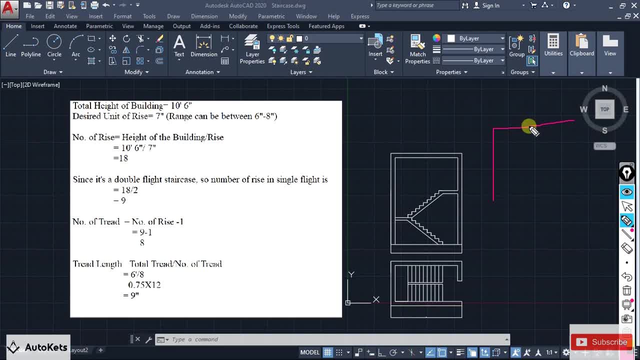 there are two things in the single state of this one, the where you rest your foot is a tread and that, hi at the elevation of this footrest, is the rise. So these are the two important terms, or parameter that is calculated in staircase design. So here we have to provide you, we have to provide we know the height of the building where we have to reach, and then the desired unit or desired height of the rise. 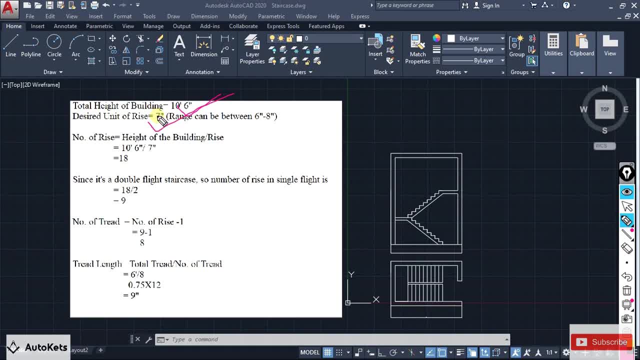 So it ranges between 6 to 8 inches. So here we have taken 7 inches and accordingly it has calculated the number of rises, or the number of rises that required to reach that particular height, as well as the number of threads. So if you know the number of rises value, you can obviously create that thread. 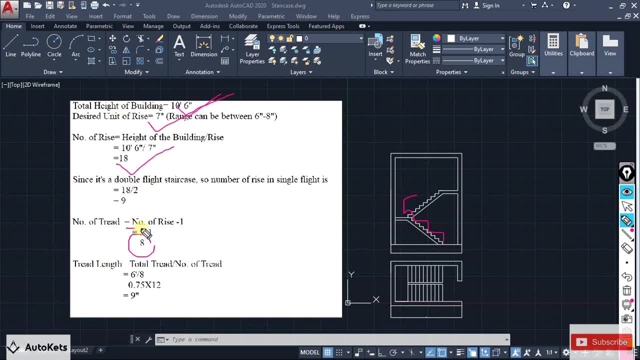 It's a thread, well, number of threads. It is a number of rises minus 1, which is 8.. Here it's a double flight staircase. It means that it is divided into two parts, So it's the number of rises per part is 9.. 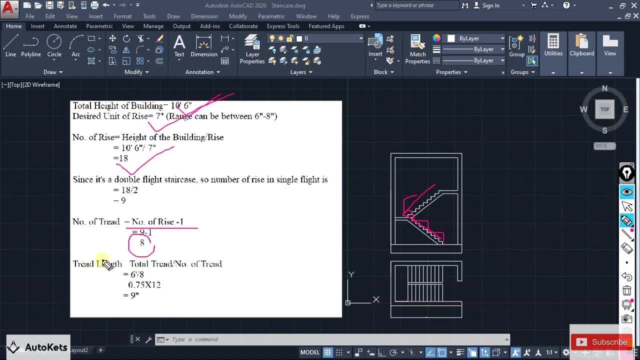 So number of threads becomes 8.. So this much calculation required to create this there. But we are going to use our list program to automatically to automate this process. So I'm going to start my chat GPT and I'm going to tell chat GPT to create the list program for me. 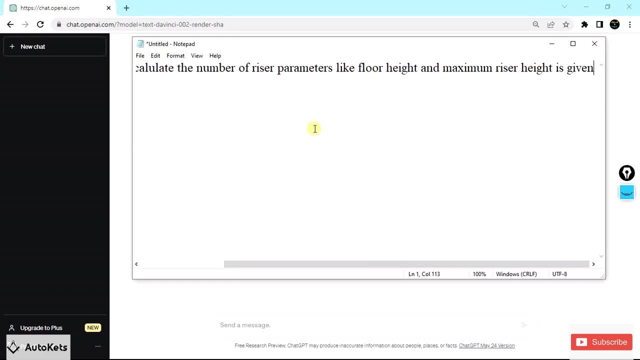 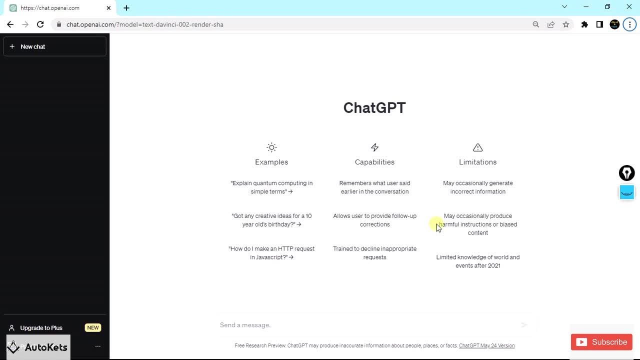 So I have the query. So I have just written a query in the notepad, So I'm going to copy this Press select copy it. And I'm going to paste this in This query box. If you don't know, if you have not used chat GPT yet, this is how the interface of chat GPT is. 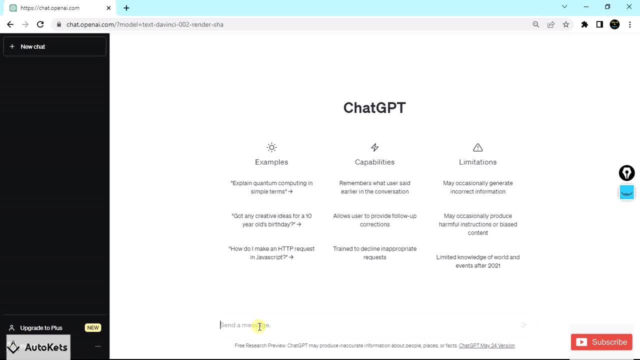 This is the place where you have to write a message or a query And, accordingly, chat. GPT will perform its AI operation and will going to provide you the result. So I'm going to paste it over here. And this is the query, which is: write an auto list to calculate the number of rises- rises- 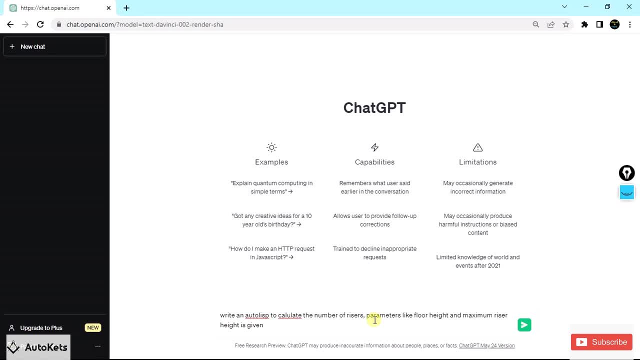 You can say that I'm going to make it comma. parameters like floor height and maximum Riser height is given, So we have to calculate the number of rises. Once we get the number of rises, it's very easy to calculate the number of thread, which is number of rises minus one, so that we can automatically do that. 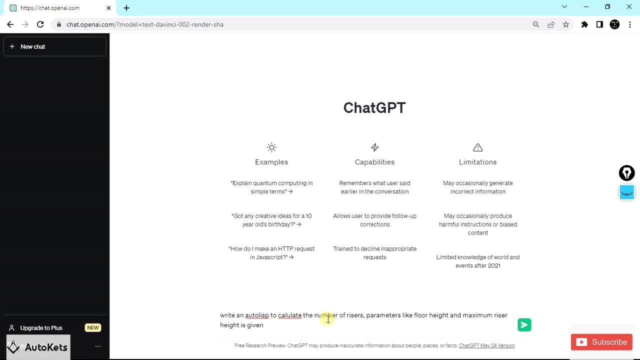 But here it will automatically. it will going to create a program that will going to calculate the number of rises, and parameters like floor height and maximum riser height is given. Was your query is done. You have to paste this button over here, which is send message, or you have to simply press enter button. 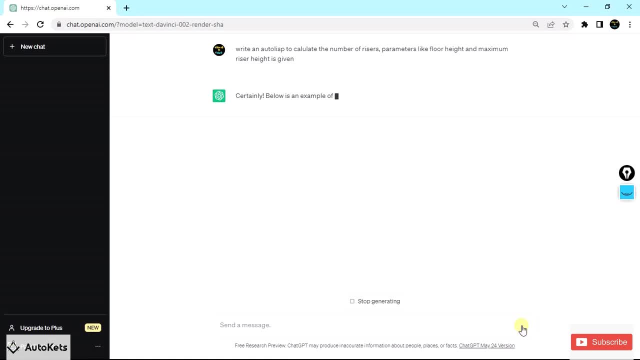 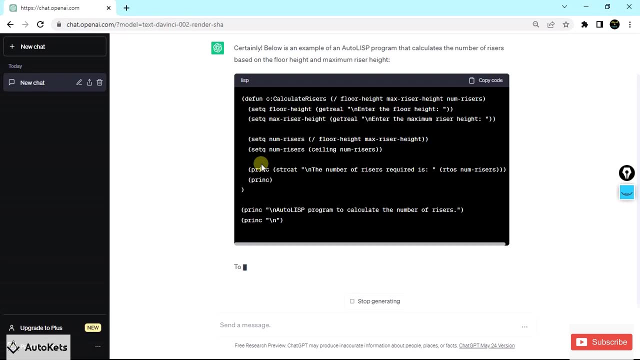 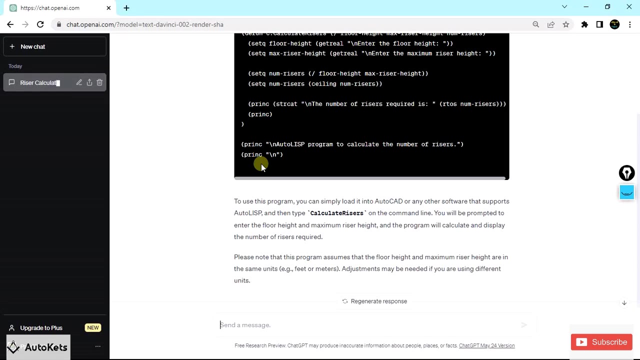 And it will going to do the magic. It will going to help you in creating that program. So here you can see that it has written a program in a certain black window And it will also going to tell you everything about the program. So if you want to read these things, you can read it like how it has created the program. 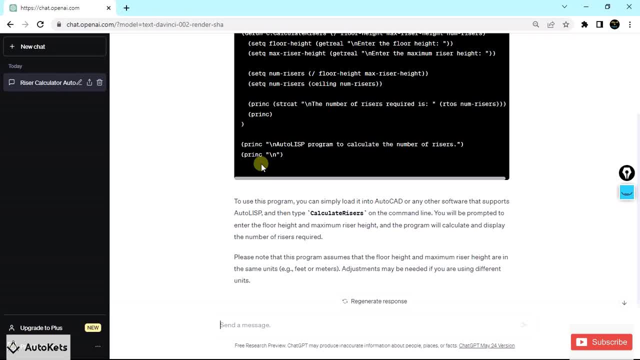 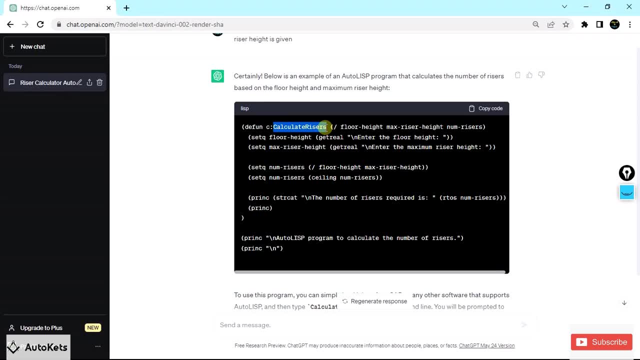 What will going to be prompted when this program is going to run. So all of the things are written over here. Just go through this And here you have to write a note. One thing, that what will be The name of this program. 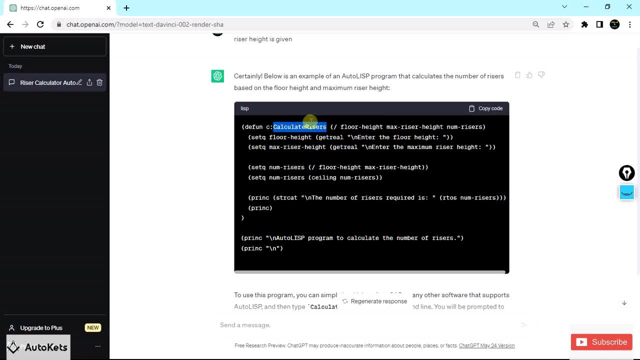 So the name of this program is calculate risers. So this is important. This is the name with the help of which you search this program. So I'm going to copy this code And once this copy code is copied, you don't you have to do this process, which is I'm going to start my AutoCAD. 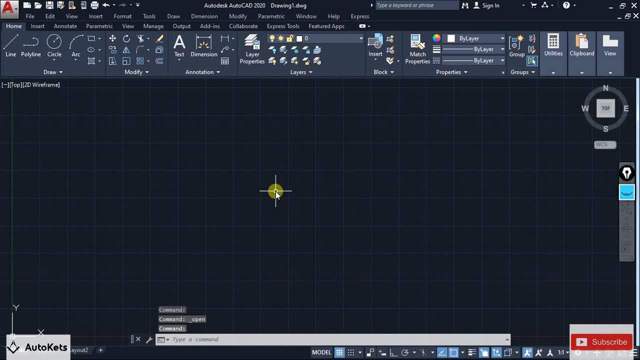 And I have a fresh page of AutoCAD over here. You can see that here I'm going to type free lisp in command box, which is a virtual lisp, So let me just write it And here you can see that free lisp will going to be available. 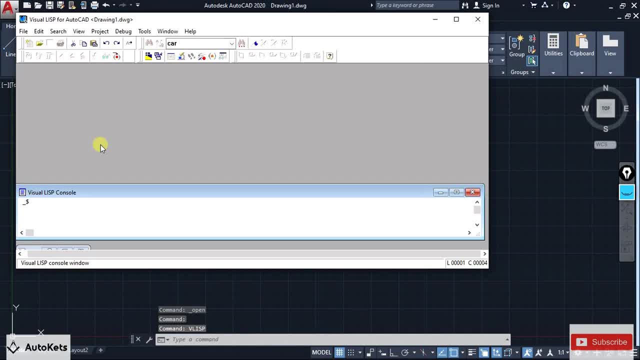 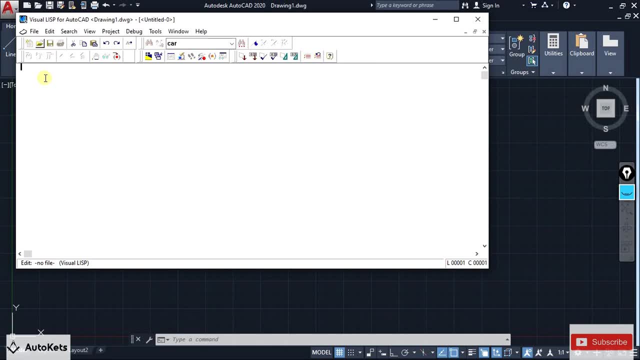 Click on this and a free lisp dialog box will going to be available. So here you have to click on this file- new file- and the first page of this lisp programming will going to open. Just paste the command over here. So I paste the command over here. 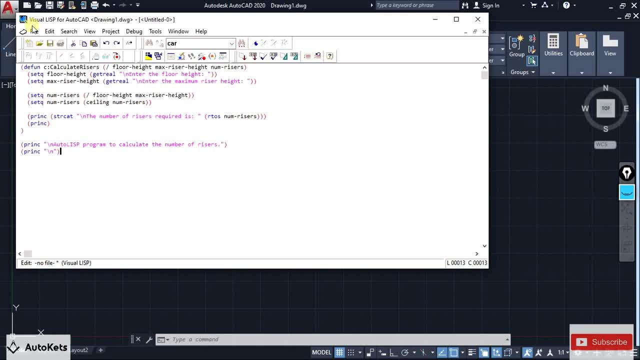 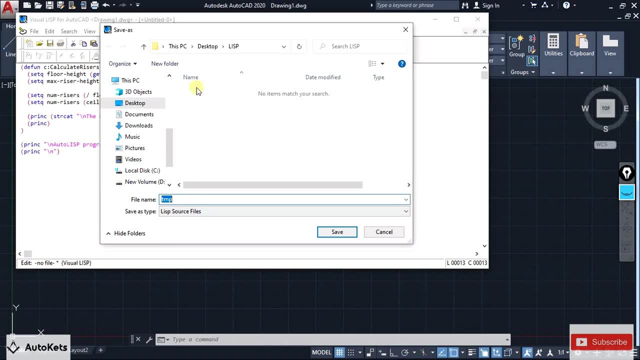 You can see that, And once I paste this command, I have to click on this file, and then I'm going to click on the save as, or save basically, And here then you have to save this in a particular folder. It will, It's going to be saved as lisp source file. 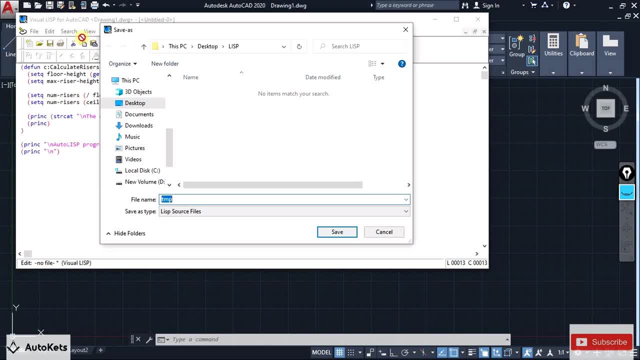 So this is what it will. This lisp, you can say that over here visual box- will going to do for you. It will going to save that file in the lisp format. name it as if you want, like I want to name it as there. 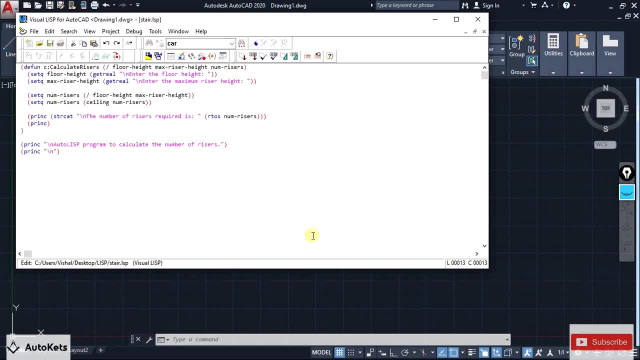 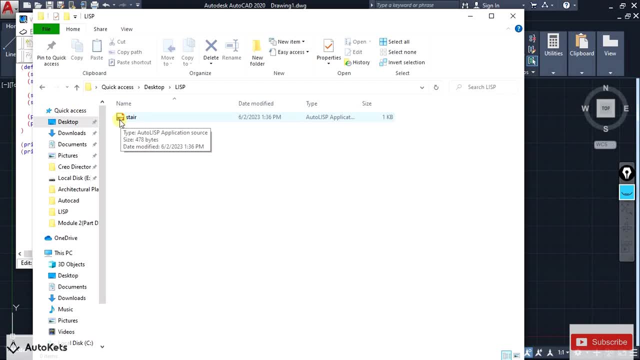 So once I named it, I can press the save button and this will going to be saved. I have the folder open, so you can see that now it has been saved over here as a lisp file- lisp. Now, what I have to do I have to just open that folder again and then I have to just simply just click on this, drag it and drop it on your AutoCAD file. 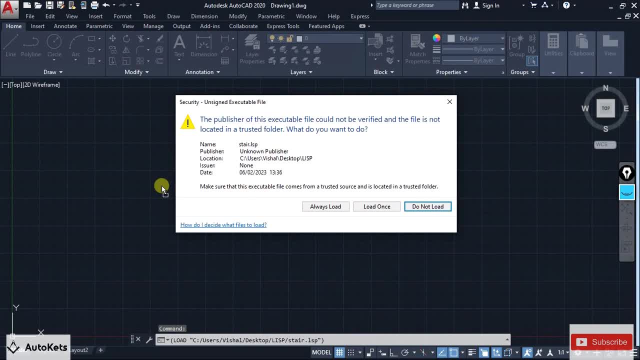 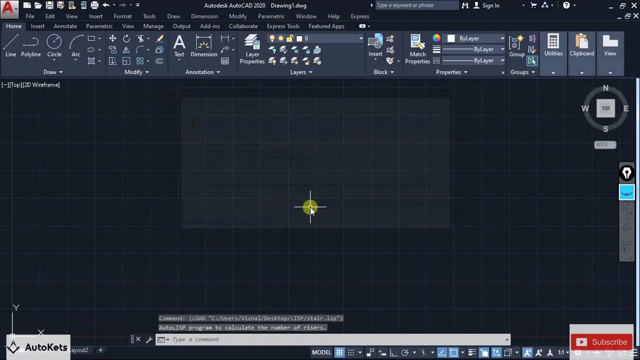 So I'm going to drag it and I'm going to drop it over here, And once I have done that, you can see that another dialog box will going to open here. You just have to press the always load button and you can see that this program will going to be load up. 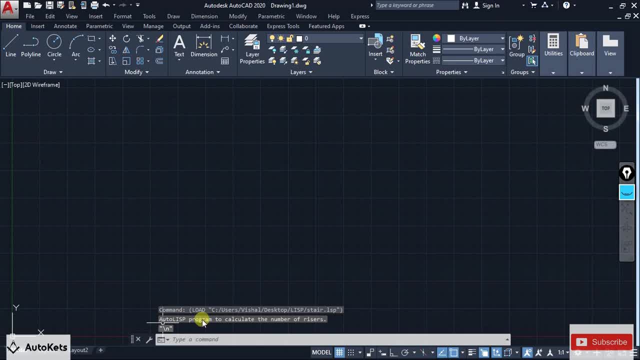 So here you can see that it has it in that auto list program To calculate the number of rises. now remember the name of the program. You have to type it over here, which is Cal, and you can see that it will automatically going to provide Cal all the things related to the Cal, like Cal tool, calculator. 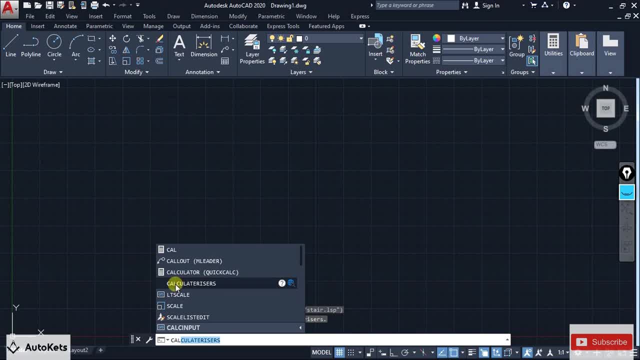 And this is what custom made program that we have made, which is calculate riser. Just click on this and then it will going to ask you for the floor height. Just provide the value, which is then right now, we haven't refined this program. 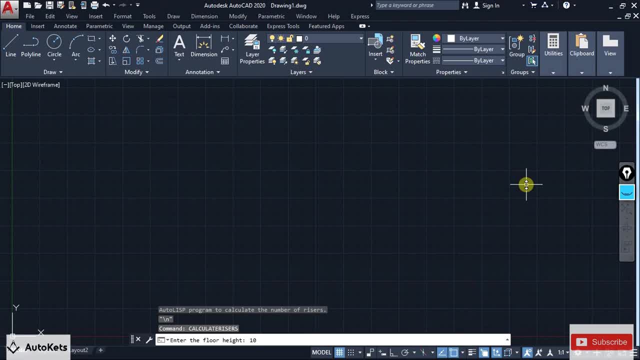 It is. It's not asking you for any unit, but later on we are going to see that also. I provided the floor height as 10, just may press enter and then it will going to ask you for the maximum riser height. We are going to take it seven inches again. 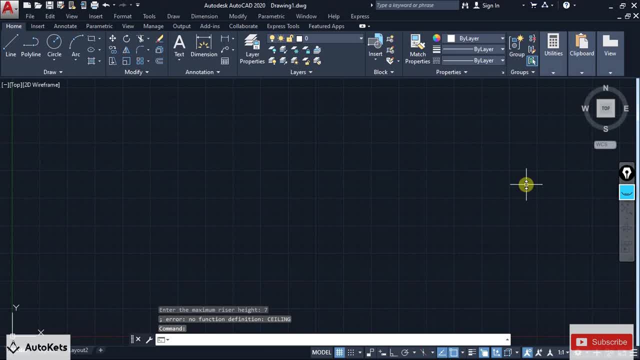 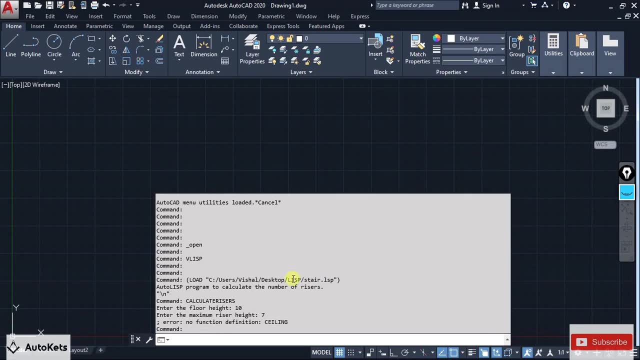 So I'm going to write seven over here. just press enter And here you can see that the error is popped up, which is error: no function definition ceiling. So there is one function that this program contains, which is ceiling, that is not available. 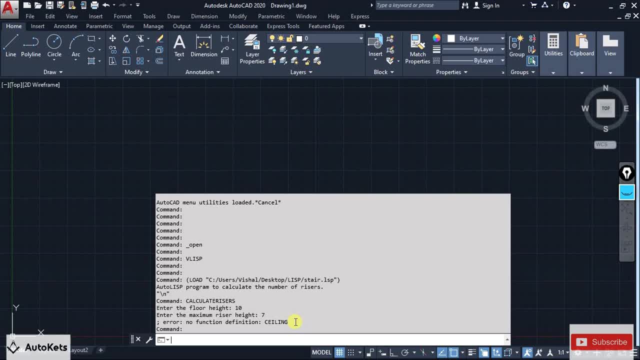 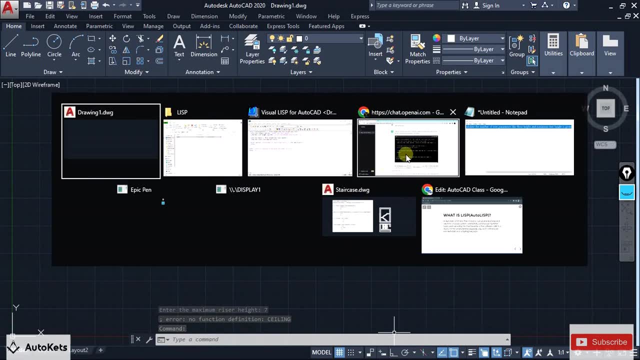 So we have to tell chat GPT that you have created a program That is showing up an error. So you have to just copy this error over here. just copy it, and then you have to open the chat GPT again. So where's my chat GPT? 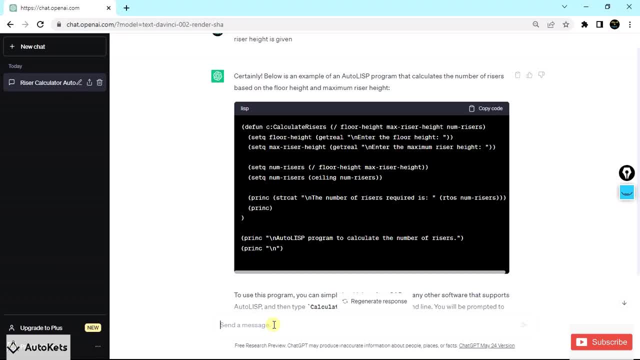 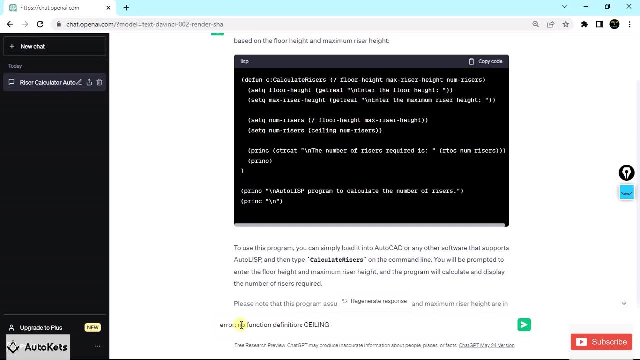 So this is my chat GPT and I have to paste this message over here. So this is the power of chat GPT. You can just talk to this as a human. So I'm going to paste this one and I'm going to just make it enter again and it will again going to tell you that it will going to apologize for that. 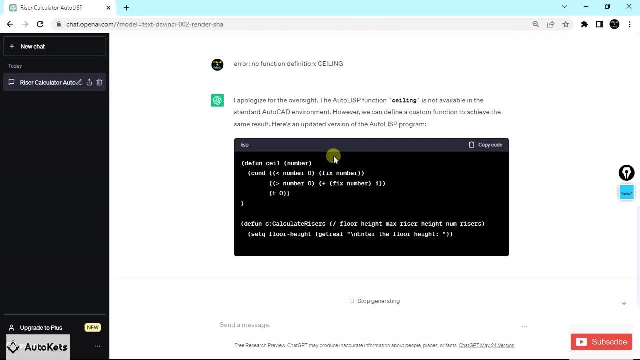 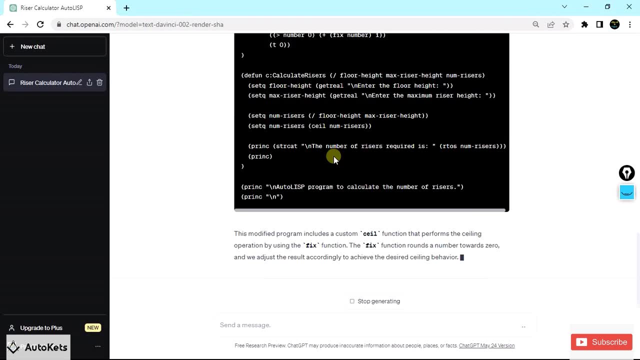 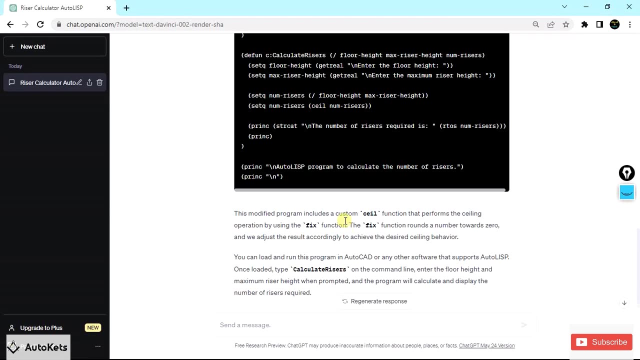 Because if this function is not available, so it is preparing a new code that does not contain this function or the updated form of this function. Once it has created the program, it is also going to tell you that what are the problems that it has fixed, like it has changed the function. 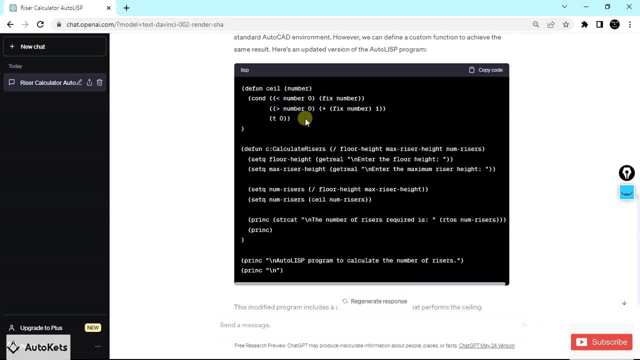 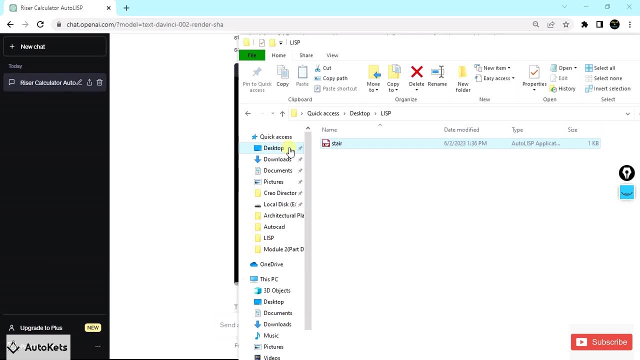 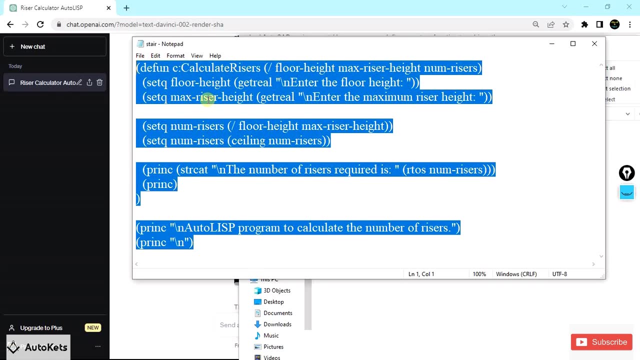 And now this program is that it has created this fun program like this: just copy this again, and then you have to open that list file. Okay, Just double click over this, and then you have to select all this and instead of in place of this program, you have to place the fresh one, and this is the correct program again. 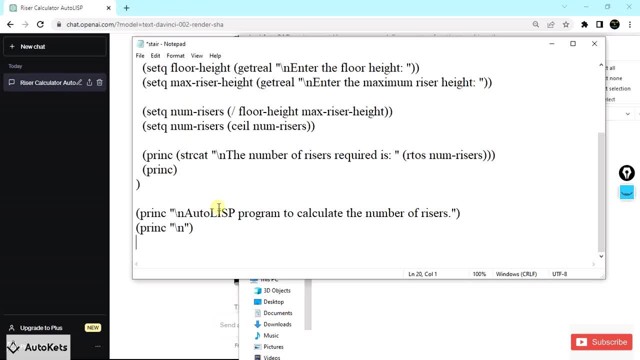 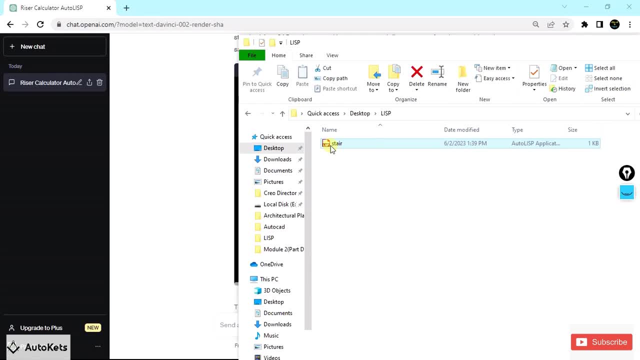 Then just press the control plus S button and that's it. you don't have to do anything. Just press the control plus S and this program will again going to be saved in the same same file again. Just go for the AutoCAD, just drag this program again. 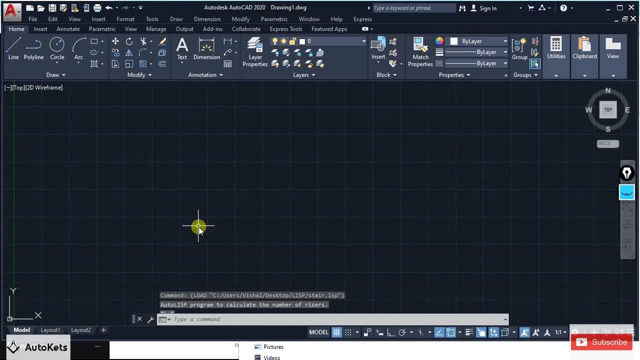 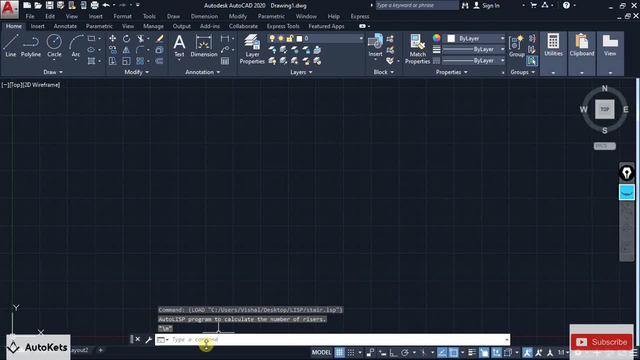 Okay, And then you have to write the name of the program again. Again it will going to be open. Again it will going to ask you for the parameters. provide that parameters And you can see that the number of rises requires is two. 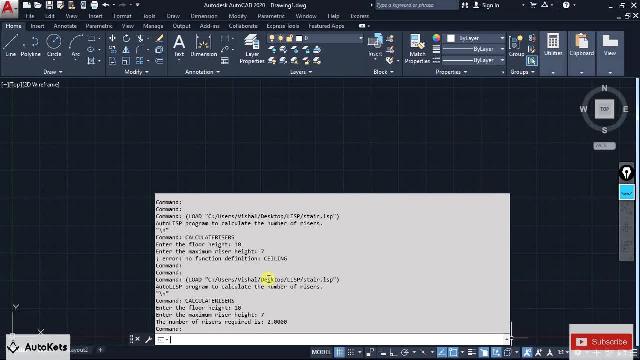 So here again, one thing: we have to see that we have taken the floor height as 10 and the number of riser, or 10 feet, and a number of rises. maximum number riser height is seven inches and it has created the two risers so to reach the 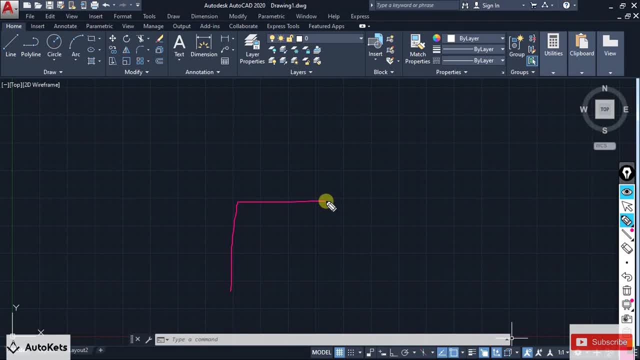 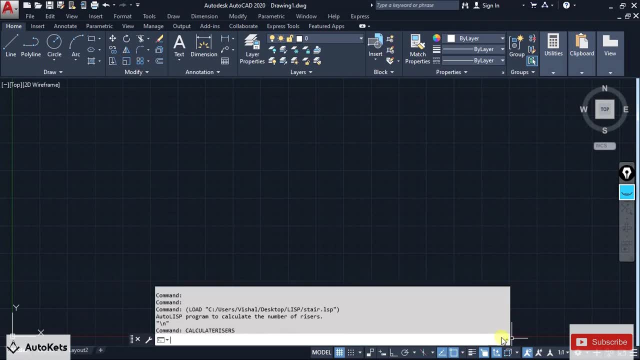 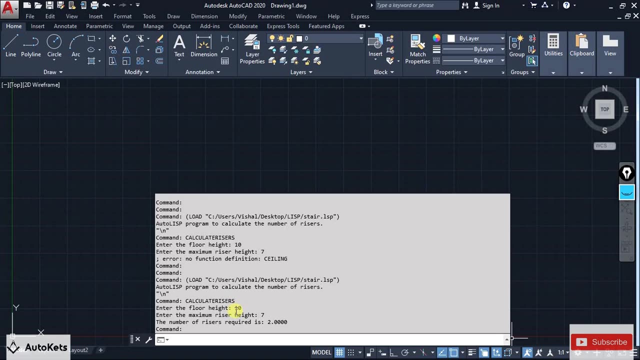 10 feet we are. we only required only two risers. it means that something is incorrect in the program and that is what incorrect is is the unit. we haven't tell the unit. so right now it is taking as a single unit. so we have to tell the autocad that here this will be in the feet and this will 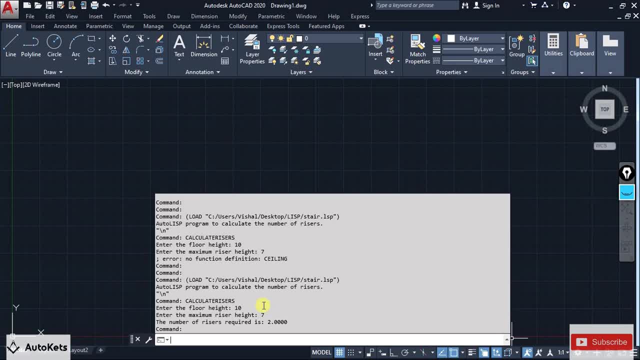 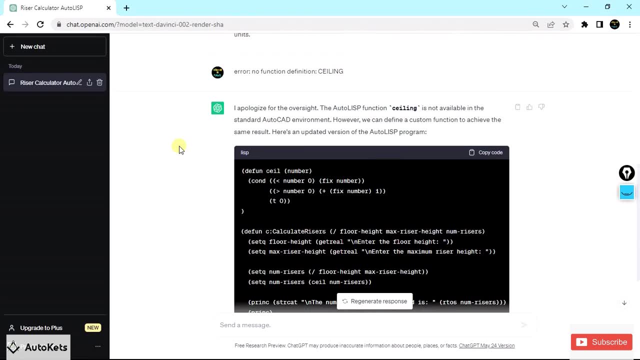 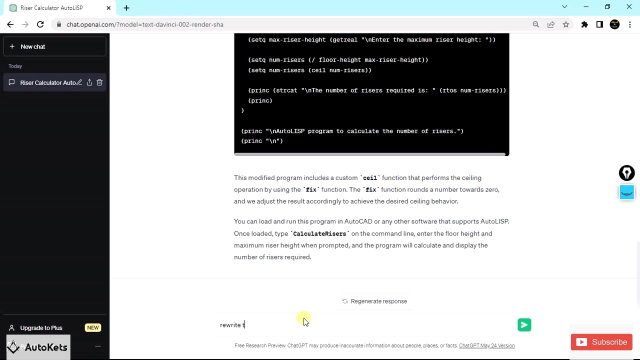 be in the inches, then only it will going to create, it will going to give you the correct value. so again, we have to update the program. so I'm going for this again and then I'm going to write a query again that rewrite this program. rewrite this program. program that with unit like floor height. 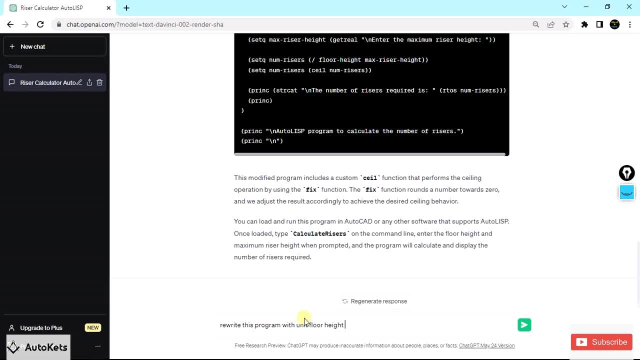 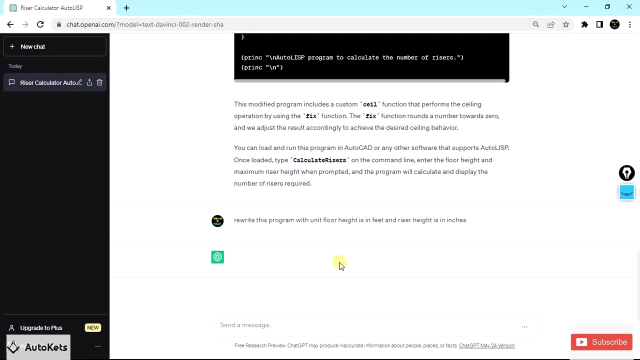 floor height is in feet and riser height is is in inches. so rewrite this program with unit floor height is in feet and riser height is in inches. so just make it okay again and let me, let just let chargpt create the program again. so it will going to take a little bit time and you have 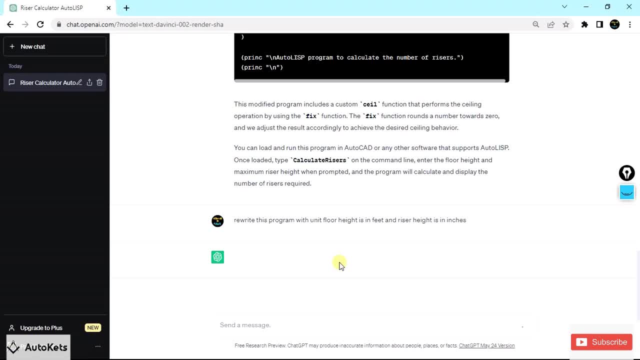 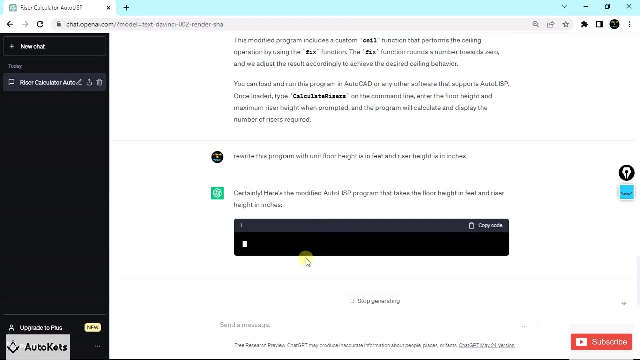 to wait for a while, okay, so here I think we have, just we have to provide a comma over here, then only it will going to. let me just see that what it is creating here it's modified that takes floor height in feet and risers in inches. so I think it has just find out what I want to ask, chargpt. 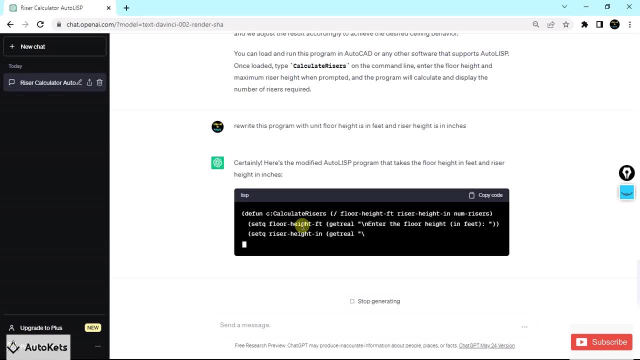 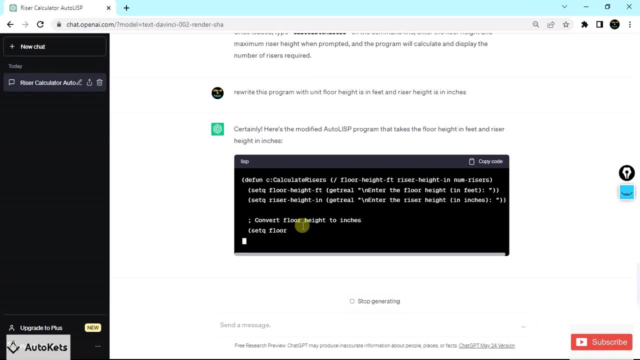 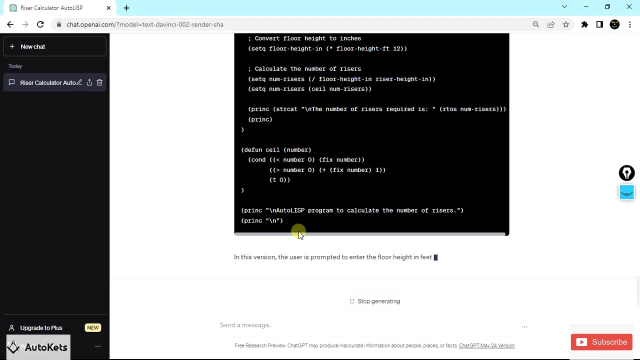 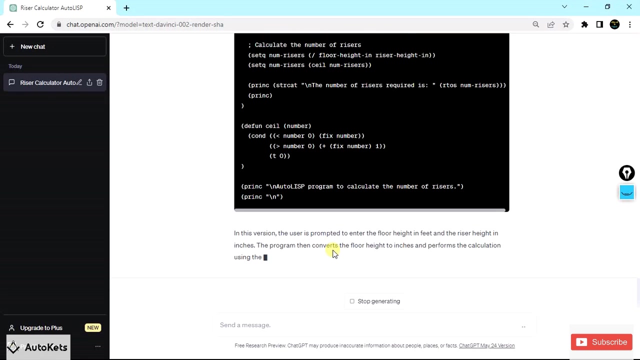 to the anybody. so it has created the program accordingly. let it create the program had. I think it is taking a letter of nothing to create it because of the processing, the processing. So once the program is over, you can see that it is telling you that in this version the user is prompted into the floor. height in feet and riser is in inches. the program alwaysieron. 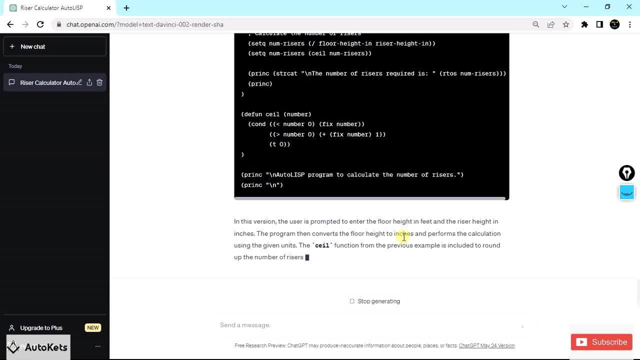 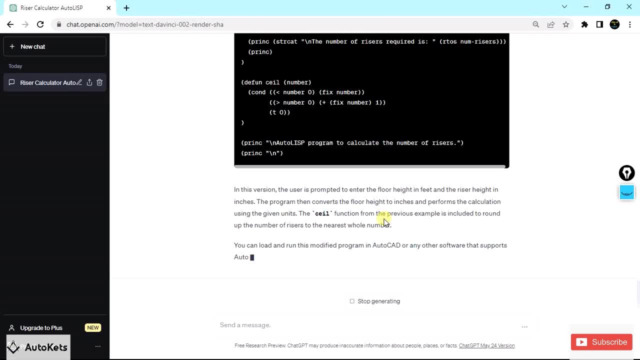 as in the feet, gives us an inches. so then, stronger. once you front to value 10, 5 inches- the floor height- into the units and it will going to calculate it. so it will going to prompt the user to provide the values in feet and inches and accordingly it will going to then convert it and 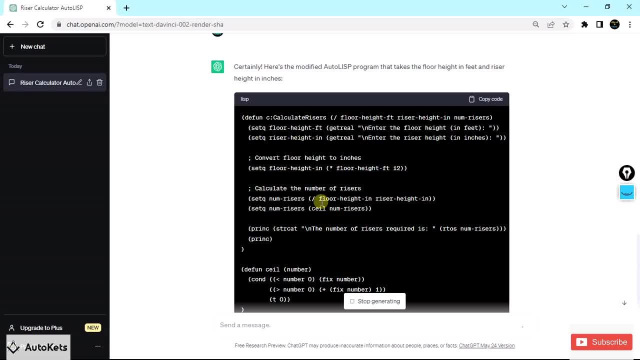 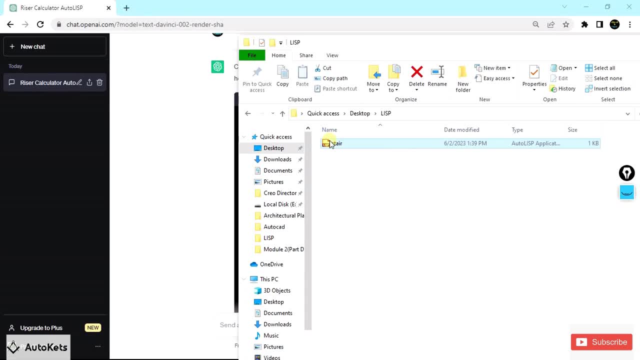 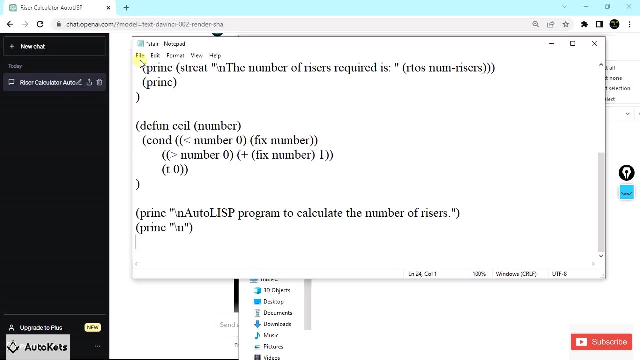 create the calculations. so once the modified program is with you, you just have to do the procedures again. just copy this code, just paste it in at this file again, just select all, just paste it, and then you have to save it again. so i'm going to press the ctrl plus s and that's it. 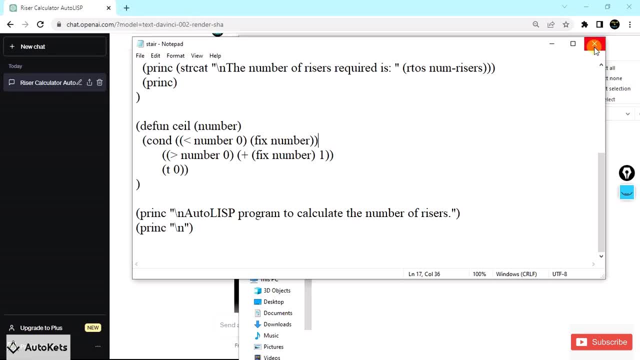 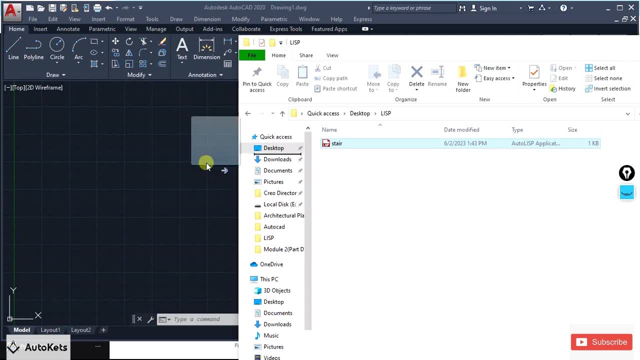 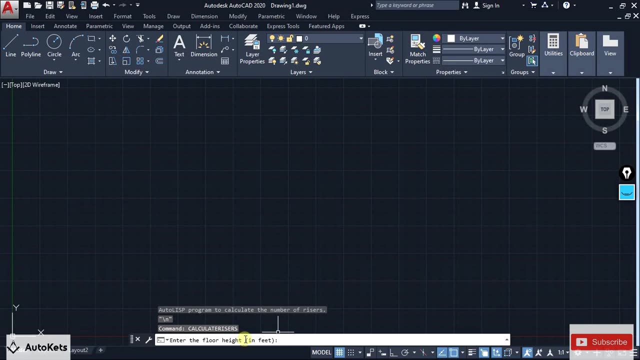 it will going to be saved. and just make sure once more. and once the it will going to be saved, you have to open the autocad again. just drag this and drop it on the screen and then again going to open the calculate riser tool and now you can see that it is asking you in the feet and inches. 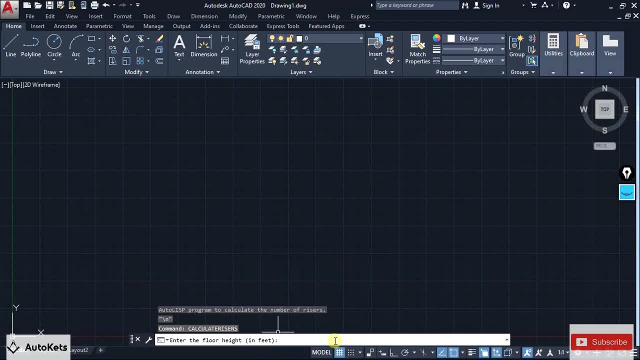 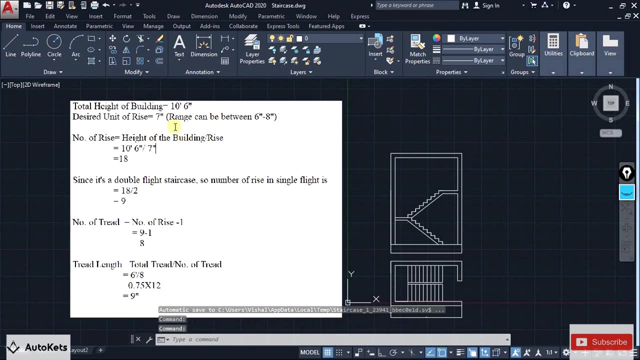 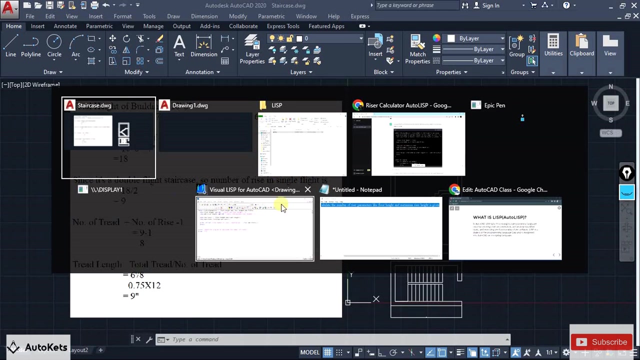 so just provide the feed value as 10 and inches- i'm going to provide this as 7 and you can see that it will going to calculate the number of rises required- is 18. so the same parameter that i have given over here. you can see that the height of the building and accordingly it has provided the values and you can see that. 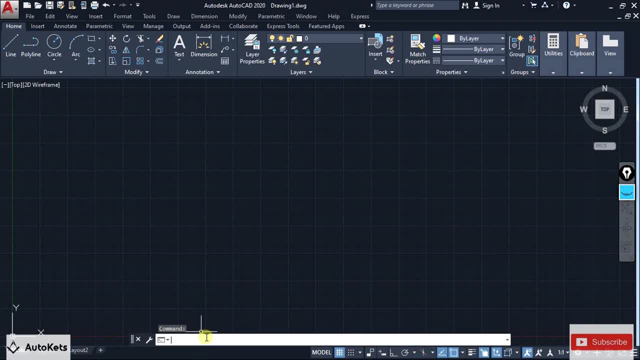 this is how you can just calculate the values. you can again open the program. just provide the values as 20 right now the floor height will be the same as the height of the building and accordingly it will be 20 feet. just press enter, the riser will be again 7 inches. you can see that in bracket it is. 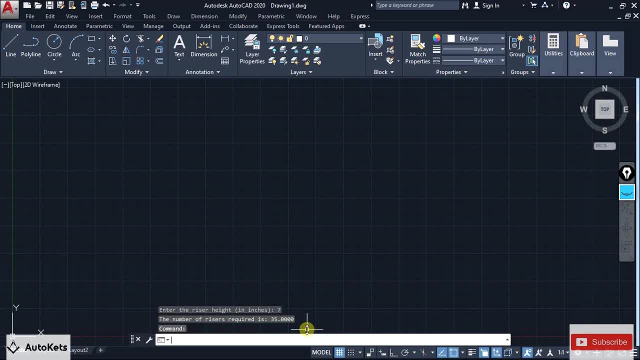 written that it is asking you in the inches. just make it enter and you can see that number of rises required is 35. so you can see that how automatically we it has created. so i haven't used my brain anywhere, i have just used a chat gpt. i have just opened the chat gpt. 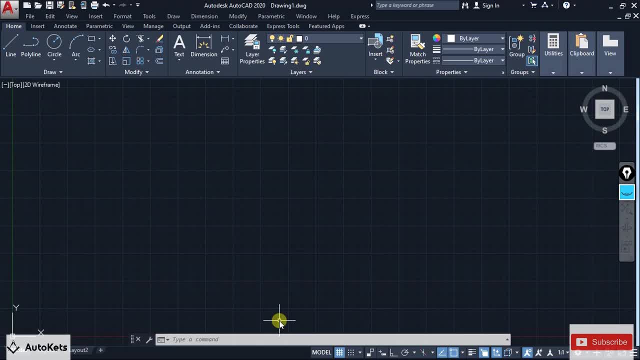 tell chat gpt to create the program. i have refined it by providing a chat gpt the parameters that i have, and then i have to just import that refined program into the autocad and accordingly it has calculated the values. so this is how you can use a chat gpt. if you have any doubt, you can ask me in. 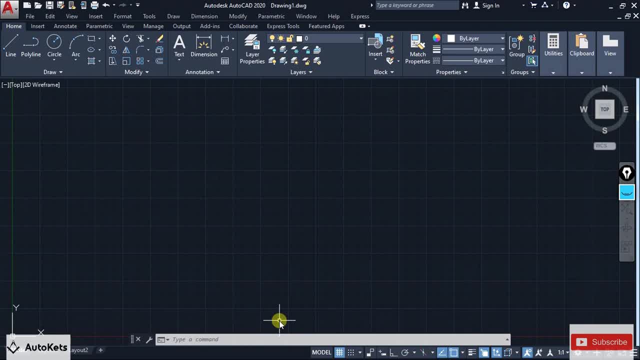 the comment and you can just create more list programs using this chat gpt and make sure that you subscribe this channel for the updates like this. thank you and catch up you in the next one. you.